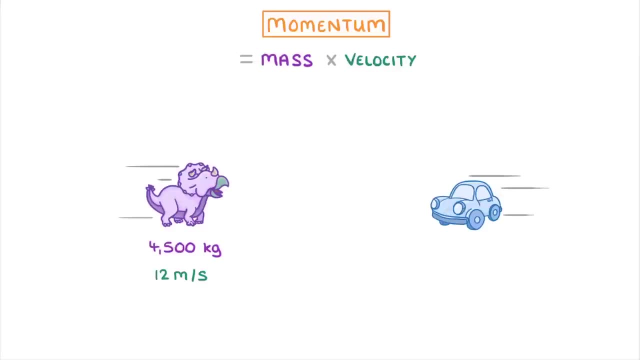 then its momentum would be 4500 times 12,, so 54,000kgm per second, Whereas if we had a 1200kg car travelling at 25m per second, then its momentum would be 1200 times 25,. 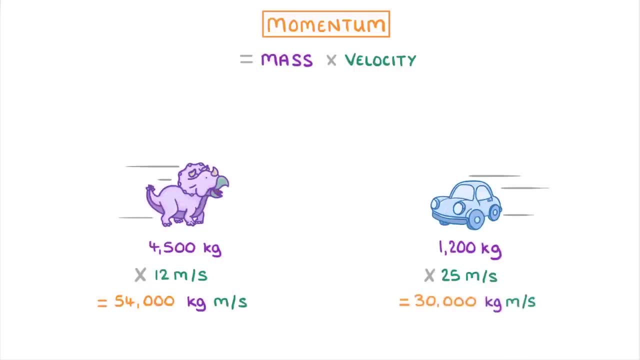 so 30,000kgm per second. An important thing to remember, though, is that momentum is a vector quantity, so it has both a magnitude and a direction. So here, if we consider the forward direction to be to the right, then the dinosaur will have. 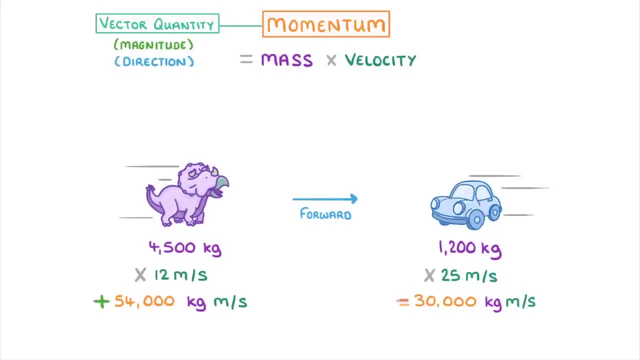 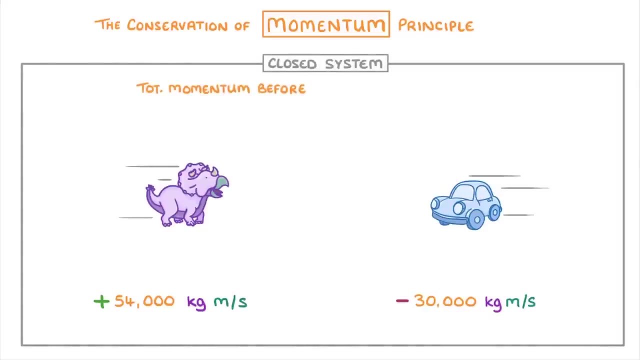 a positive momentum, but the car must have a negative momentum. The next thing to know is the conservation of momentum principle, which is the idea that in a closed system, the car must have a positive momentum and the car must have a negative momentum. In a closed system, the total momentum before an event like a collision is exactly. 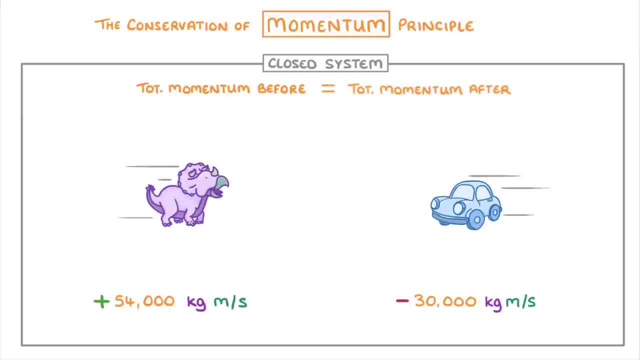 the same as the total momentum after the event. To see how this works, let's imagine our dinosaur and our car as two particles which are travelling towards each other and are going to collide, after which they'll both continue moving together at the same speed. 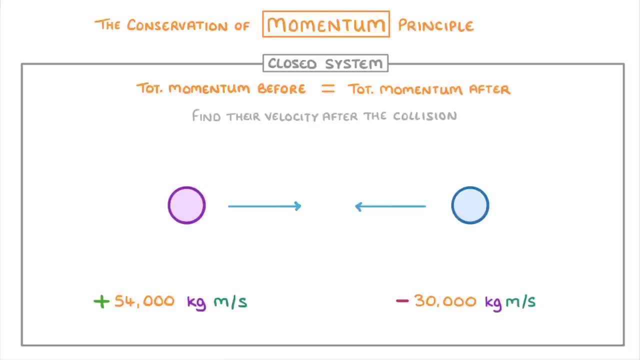 How would we find their velocity after the collision? Well, the first thing we need to do is find their total momentum before the collision, which we can do by adding together the dinosaurs' and the car's momentums, so 54,000 plus negative. 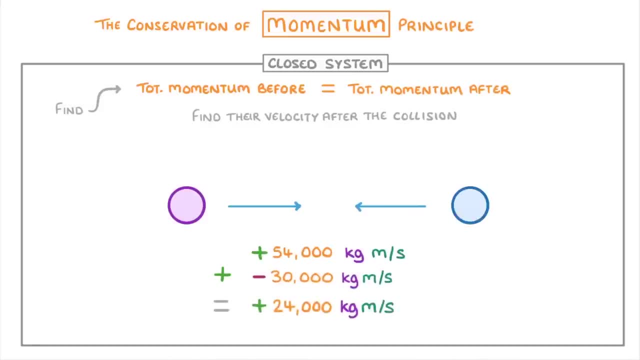 30,000, which gives us positive 24,000kgm per second. Then, because of our conservation of momentum principle, we know that once they've collided, their total momentum will be equal to the total momentum before the collision, which is 24,000kgm. 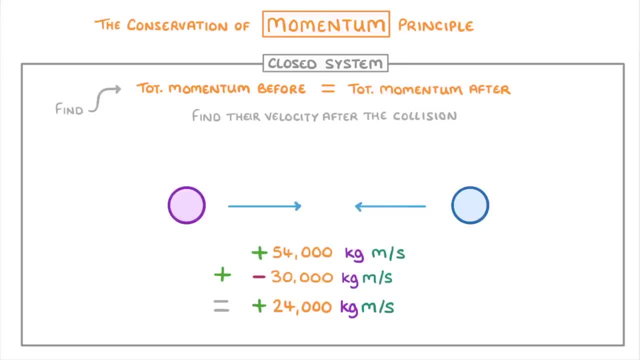 And remember that in this scenario, a positive number means that it's going to the right. So after our particles collide together, they'll both get carried to the right. because the purple one had more momentum And because they're both moving together, we can now treat them as a single large particle. 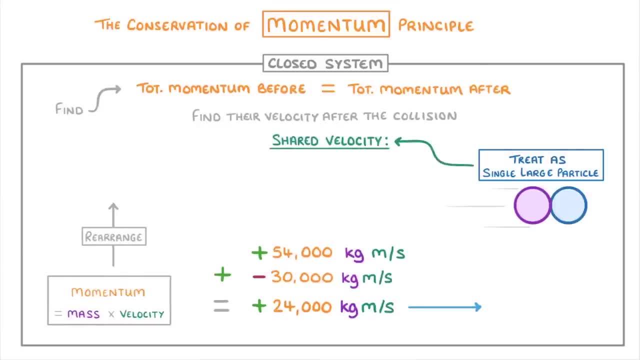 So to work out their shared velocity, we need to find their total momentum. To do this, all we have to do is rearrange our momentum equation to show that velocity equals momentum divided by mass, and then plug in the values for this combined particle. 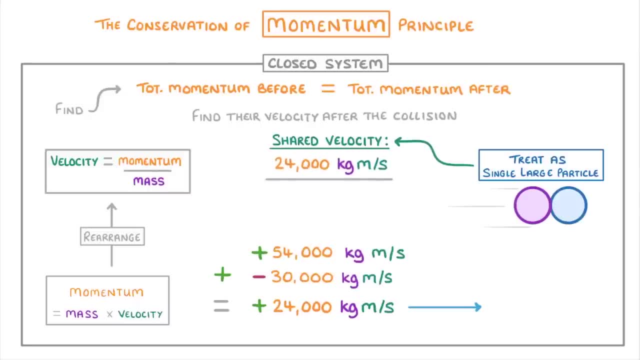 So 24,000 divided by their combined masses from before, which would be 4,500 for the dinosaur plus 1,200 for the car, so 5,700kgm, Which gives us a velocity of 4.4m per second to the right. 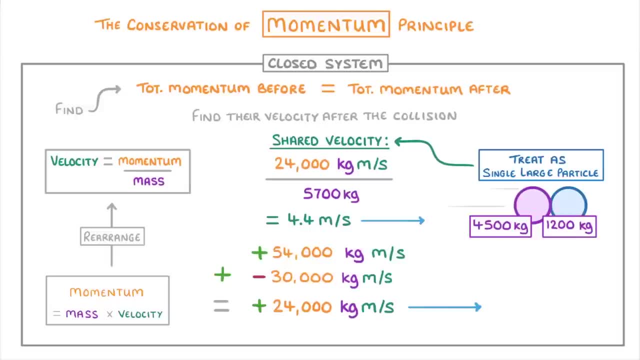 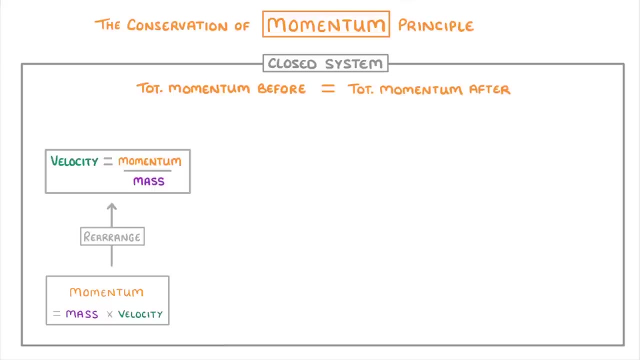 So basically, after the dinosaur and the car collide, they'll both continue moving to the right at a velocity of 4.4m per second. Now, in some circumstances, the momentum before an event might be zero, like it is for stationary. 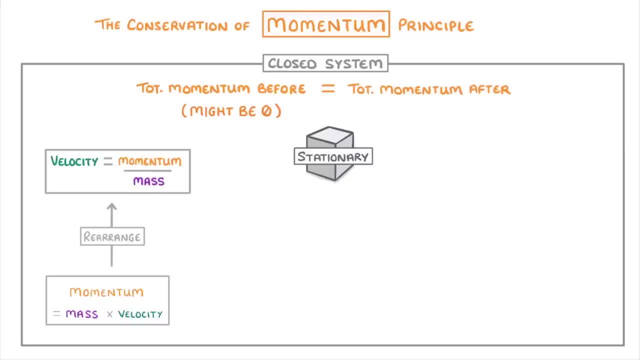 objects Which don't have any momentum because they're not moving, And so in these cases the total momentum after the event must also be zero. For example, if we imagine a gun before it's fired, then its initial momentum would be: 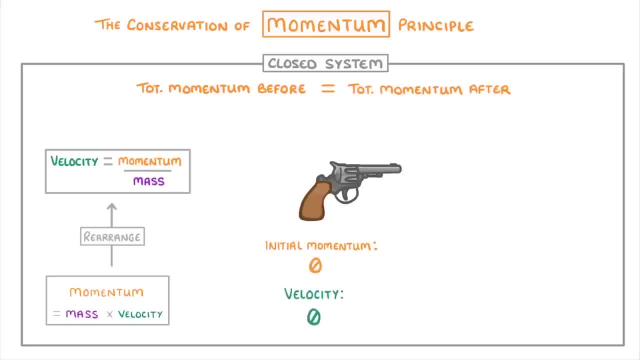 zero, because its velocity is zero. However, once the gun fires, the bullet that flies out will have a momentum in the forward direction, And that's it, And so, to compensate for this, the gun has to recoil backwards with an equal momentum. 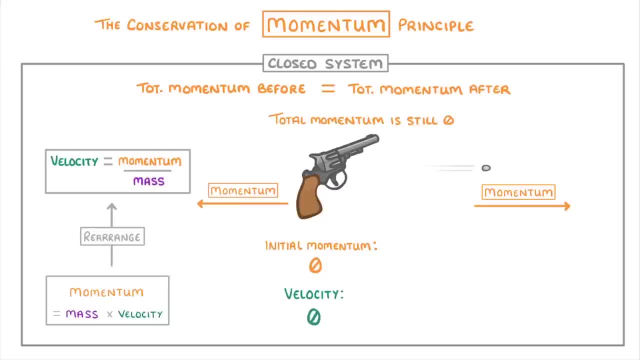 so that together, the total momentum is still zero. So if we knew that this gun had a mass of 2kg and that a 5g bullet was fired out at a velocity of 120m per second, we should be able to work out the velocity of the gun's. 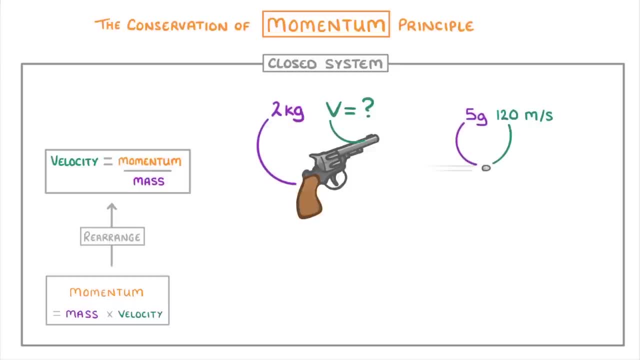 recoil. The key to this is that we should be able to calculate the velocity of the gun's recoil. The key to this is remembering that the gun's momentum plus the bullet's momentum must equal zero, because it started off at zero before the gun fired. 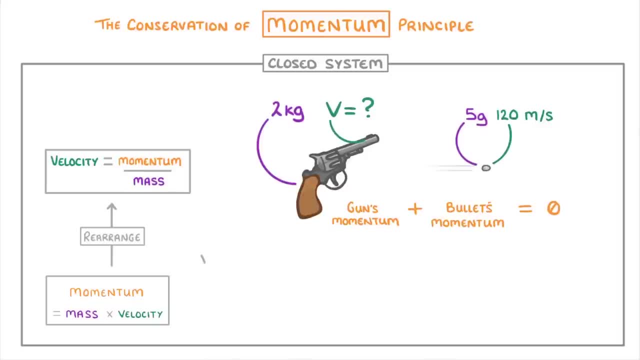 The first thing we want to do is find the bullet's momentum using this bottom equation. So we do 0.005, which is its mass in kilos times its velocity of 120, which will give us a momentum of 0.005. 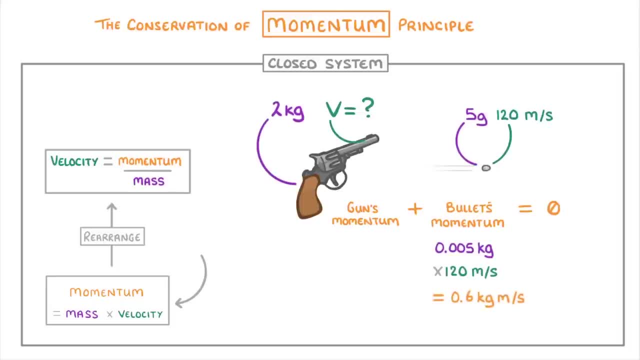 Next we want to try and find the gun's momentum. So again we just do the mass of 2, times the velocity. But because we don't know what the velocity is yet, we can just write v for velocity. So the momentum will be 2v, where 2 is the mass in kilos and v stands for the gun's. 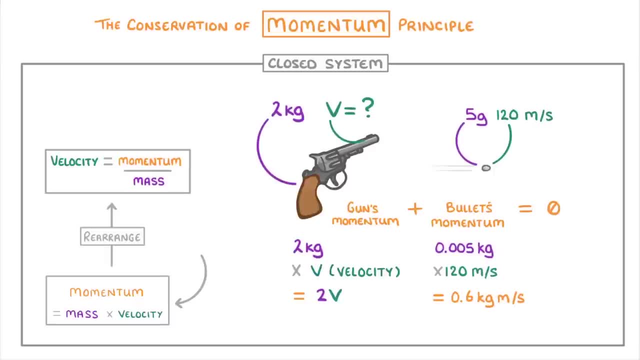 velocity, Which we're about to find. So that's it. Finally, we can use these momentum values for the gun and the bullet to rewrite our equation as 2v plus 0.6 equals zero, And then we can just rearrange this equation to find out the missing value of v. 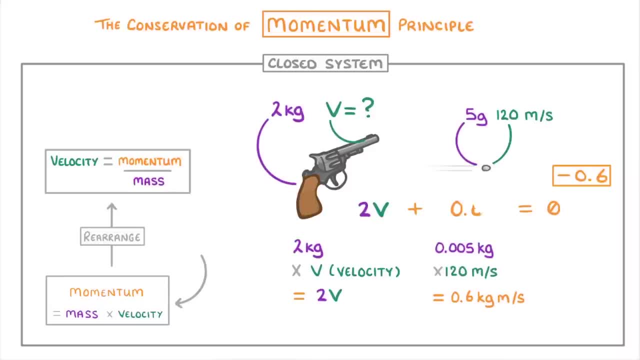 So first we subtract 0.6 from both sides, giving us 2v equals negative 0.6.. And then we divide both sides by 2, leaving us with v equals negative 0.3 meters per second, which is the gun's recoil velocity. 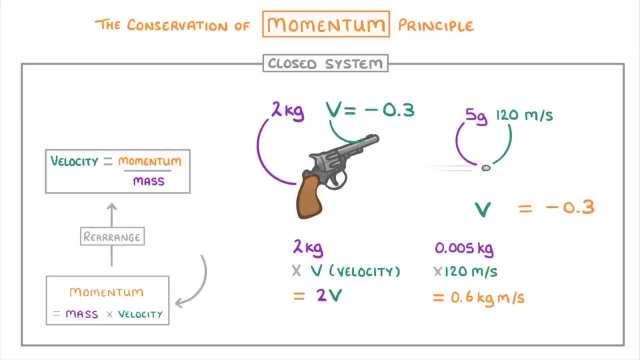 And remember the fact that it's negative means that it's effectively going backwards, Or in other words, it's going in the opposite direction to the bullet. The one thing we haven't mentioned yet is that you need to know that the velocity of 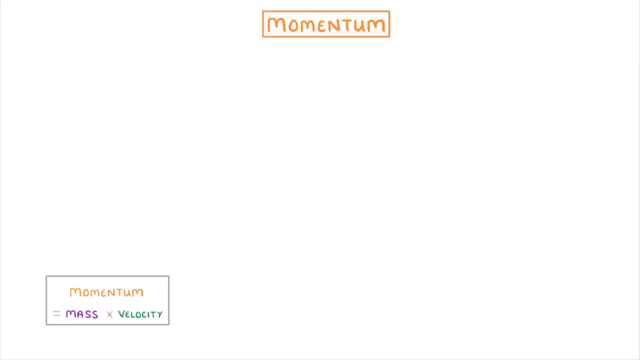 the bullet is going in the opposite direction to the bullet And that's because the velocity of the bullet is going in the opposite direction to the bullet. So we know that the letter symbol for momentum is rho, which looks like a p. So the momentum equation can also be written as: p equals mv. 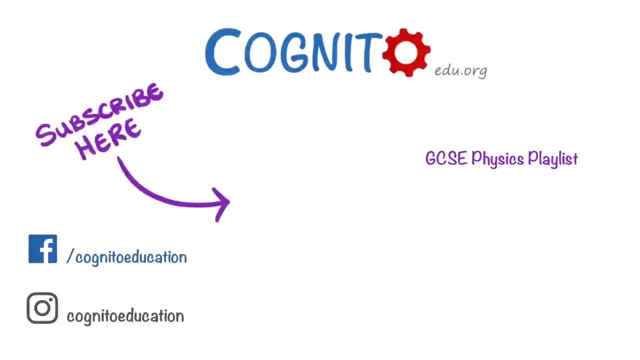 That's everything for this video, though, So I hope you enjoyed it. If you did, then give us a like and subscribe, And we'll see you next time.